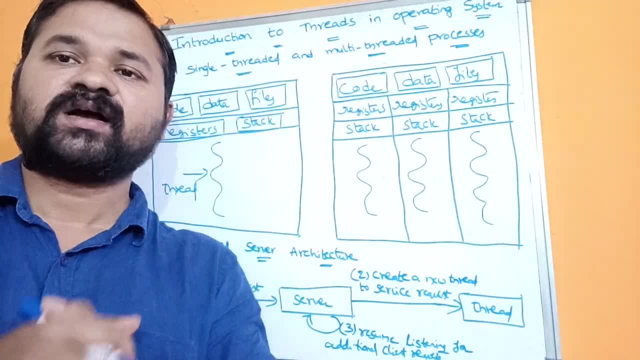 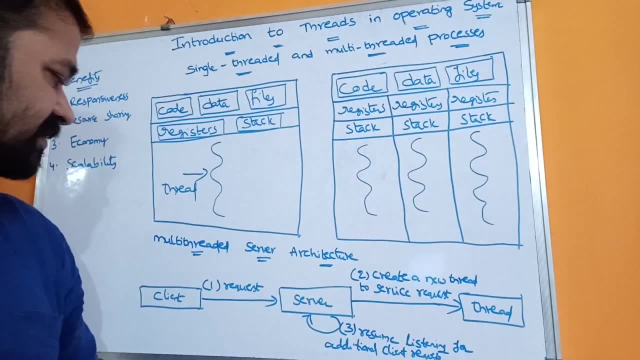 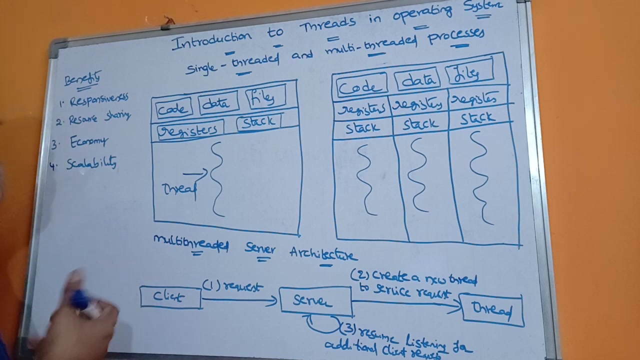 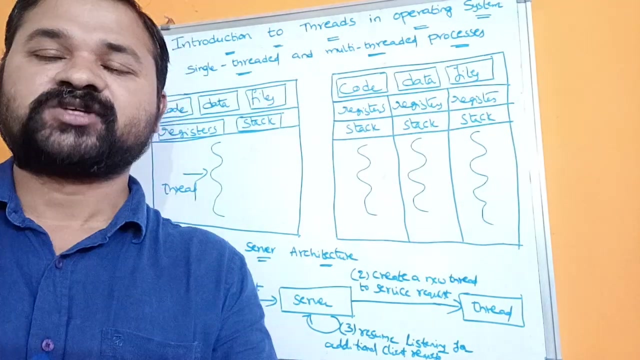 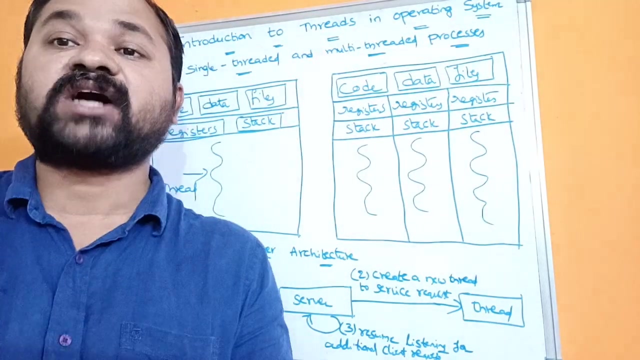 Now let's see about threads in operating systems. In this video we are going to discuss about what is a single threaded process, multi-threaded process and what is multi-threaded server architecture, as well as benefits of multi-threaded programming. So first let's see about what is a thread. Thread means a lightweight process, So that means it contains a limited number of instructions as well as thread address spaces associated with process address space. 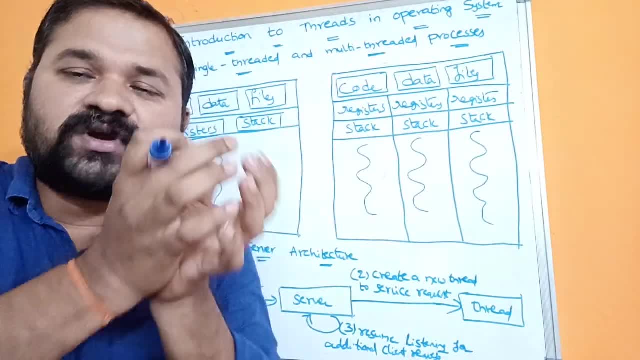 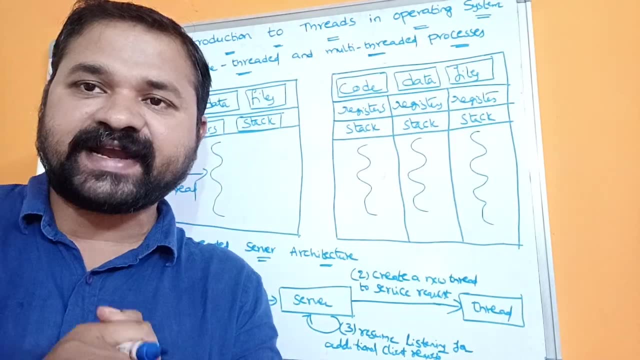 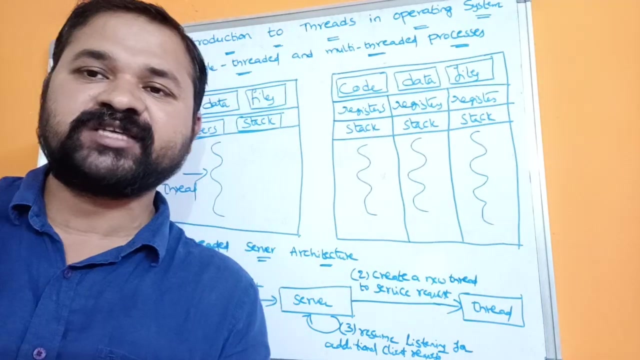 So if there is a process, then a process will be created at some address. Threads will also use those addresses. So that's why we can call thread as a lightweight process. Why? because we can call thread as a lightweight process. threads uses the address space which are associated with the process, as well as 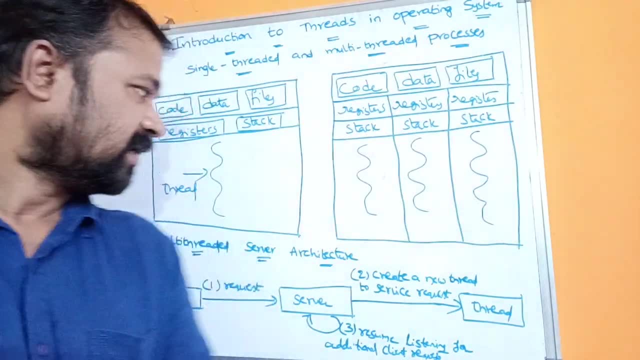 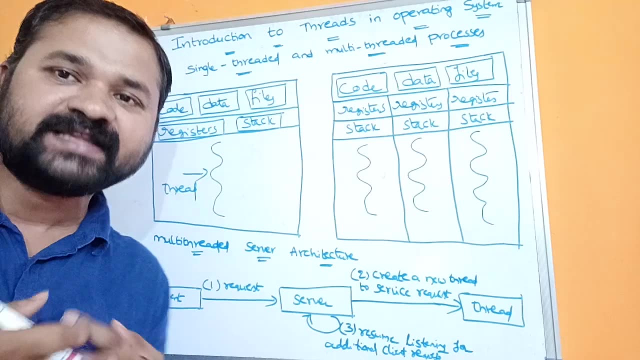 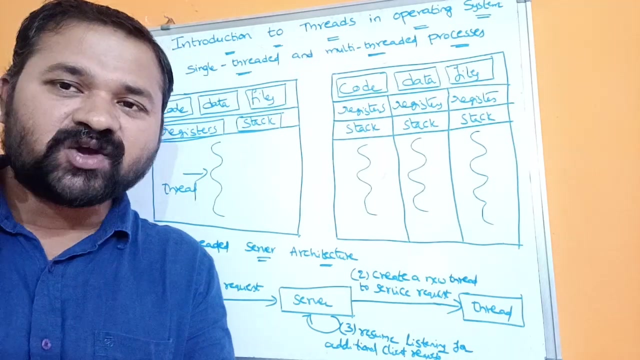 thread contains a limited number of instructions, so let's see this one. so this is nothing but a single threaded process. other areas: this diagram is about multi-threaded process. let us observe this dagger: by default, every process has only one thread of control. that means every process will contains. 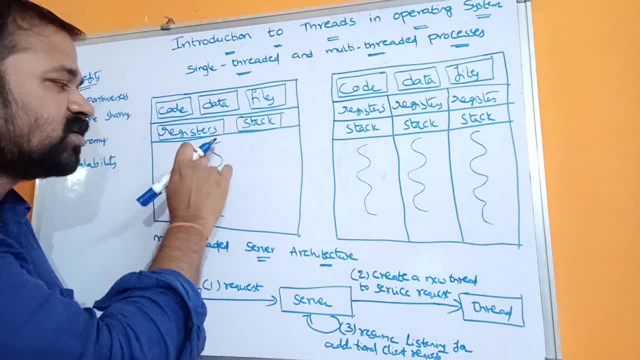 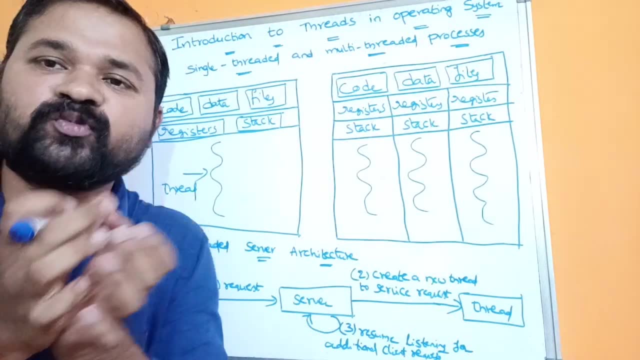 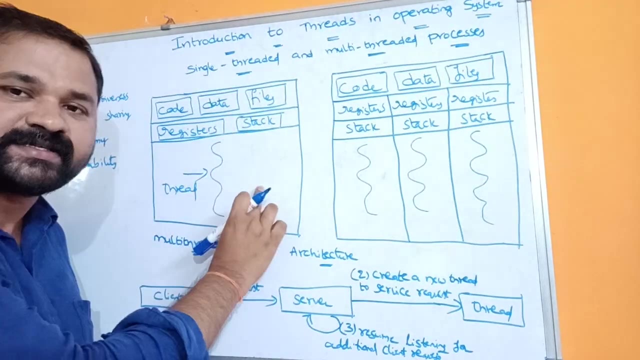 only one thread. so this thread defines flow of execution, so how the instructions are to be executed and what are the instructions to be executed. so that is about what is a thread. so here this is nothing but a single threaded process. that means this process contains only one thread. so let us observe the 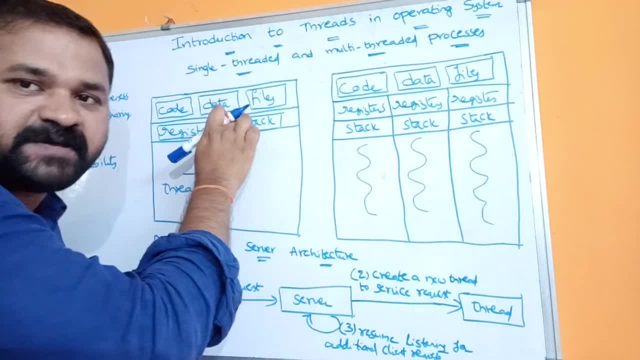 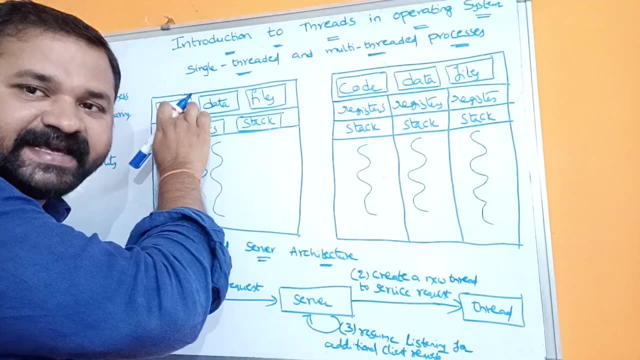 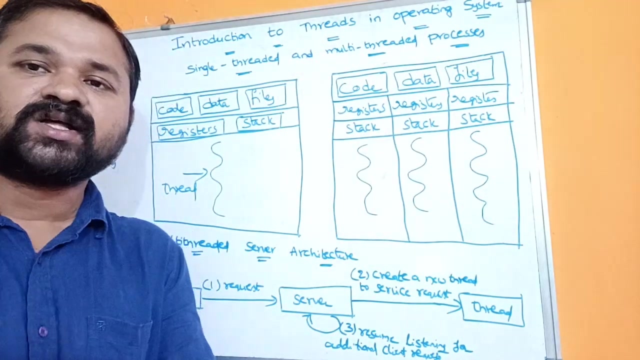 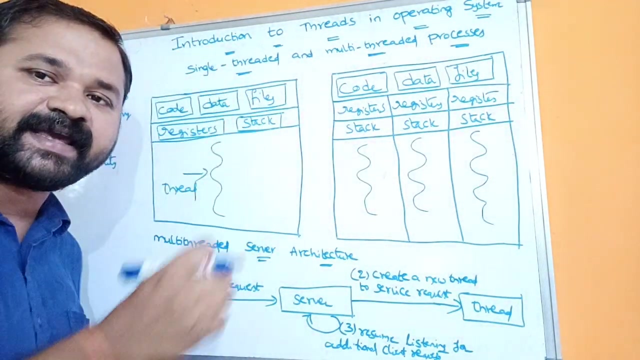 segments. here we have core segment, data segment, files segment, as well as stag segment. core segment is useful in order to store the instructions of the process. let a process contains ten statements, so all those 10 statements will be stored in the core segment. next one is data segment. data segment is: 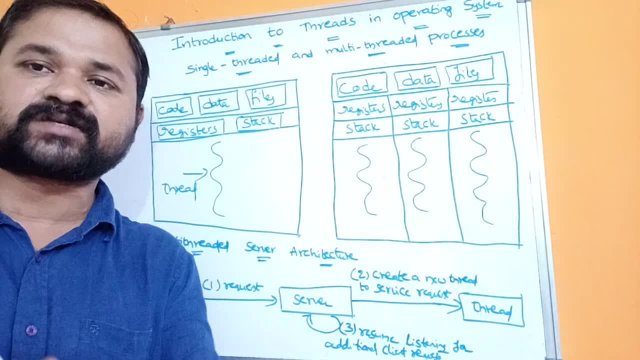 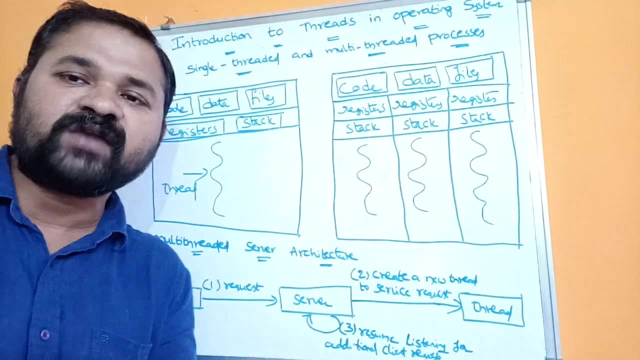 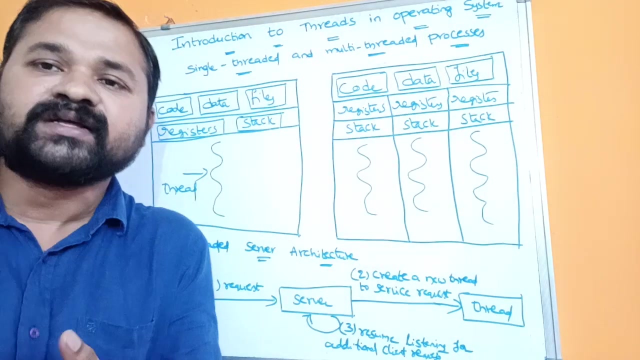 mainly useful in order to store global variables. we know what is a global variable. we can use this global variable throughout the program. so, in order to store the global variable, we use this data section and the Next one is file section. It is useful in order to store the list of files which are opened. 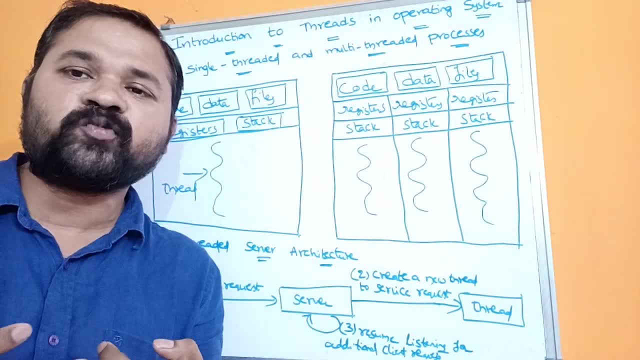 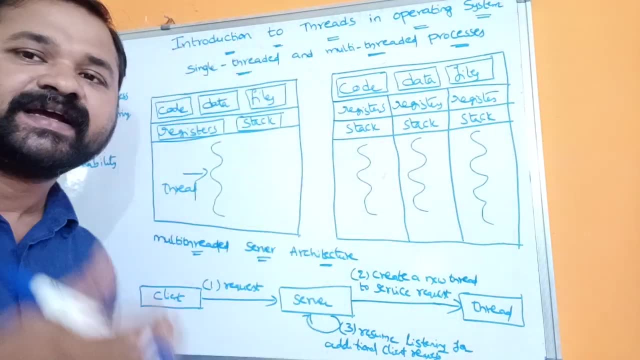 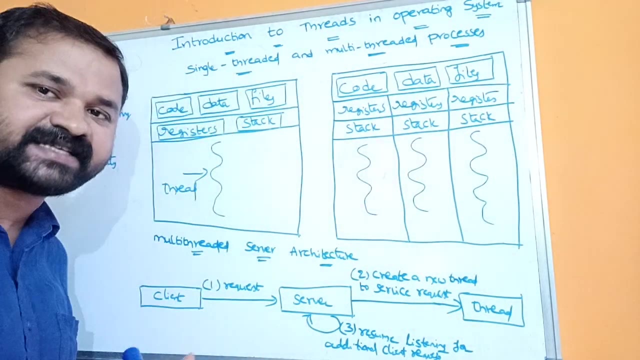 Let us assume that we have opened 5 files in order to perform our operations, So those files will be stored here. So this files section contains list of files that are opened. Next, register section. It contains registers. It contains registers like program counter, program status board, index, register accumulator. 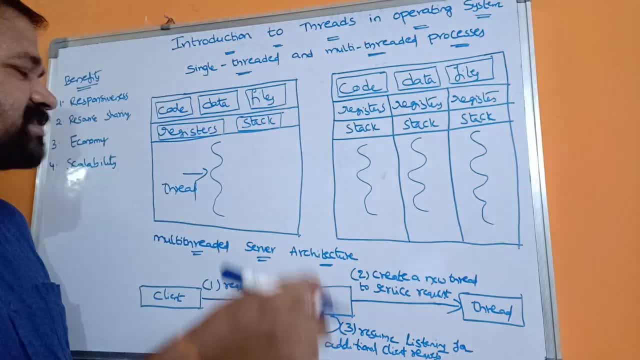 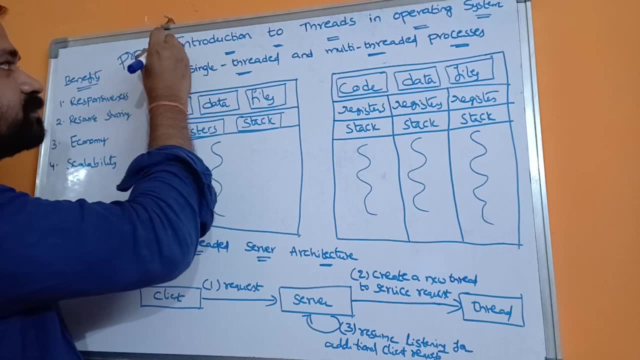 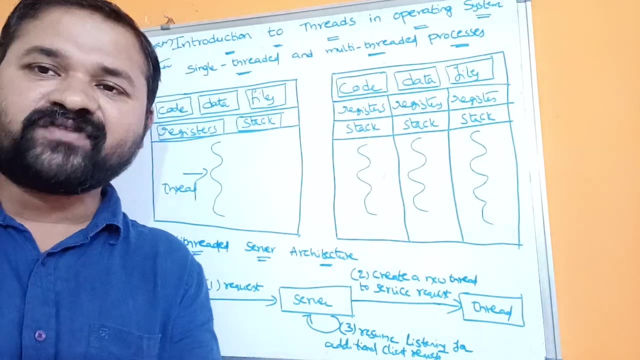 Likewise there are several registers are there, So all the registers will be stored in this section. Here mainly we use PC, So PC stands for program counter. Program counter contains address of next instruction to be executed. So whenever a process is blocked, then its next instruction will be stored in program. 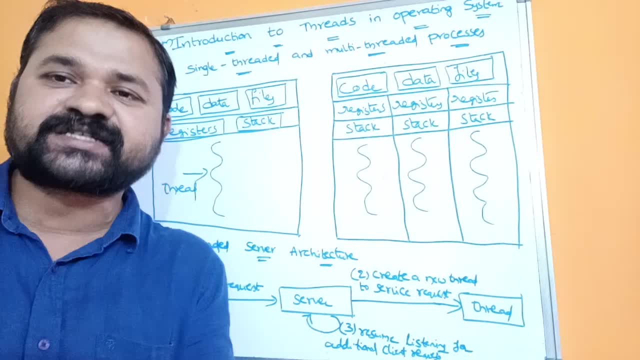 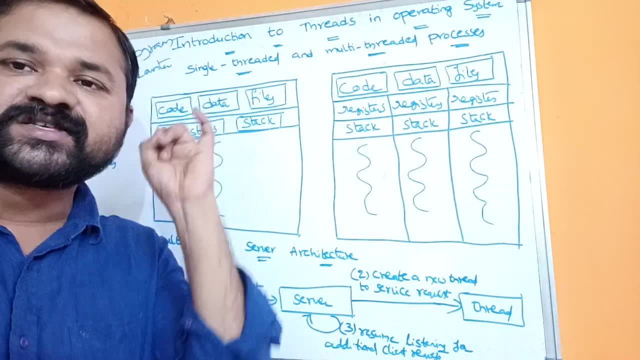 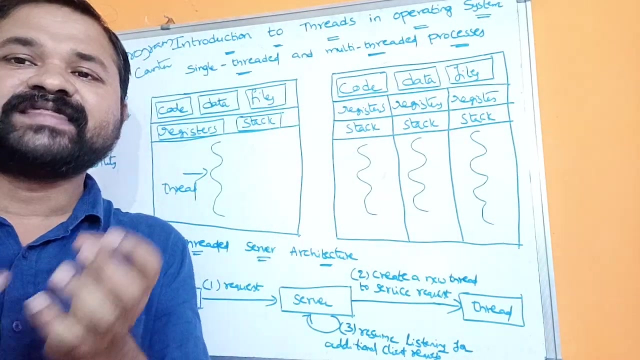 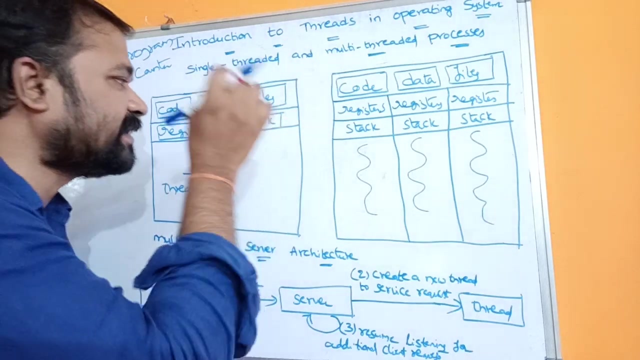 So from the program counter, CPU starts resuming the corresponding process, So that process execution will be resumed based upon the program counter. And next here we have stack section. So whenever a function is called, then the parameters of the function as well as the local variables which are declared in that function will be stored in the stack section. 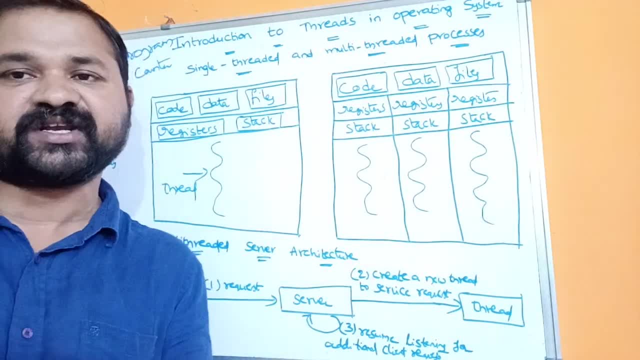 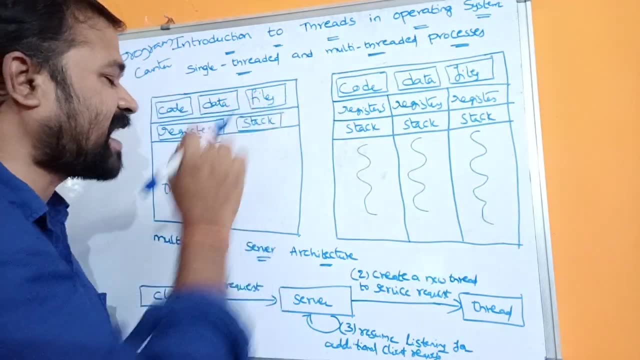 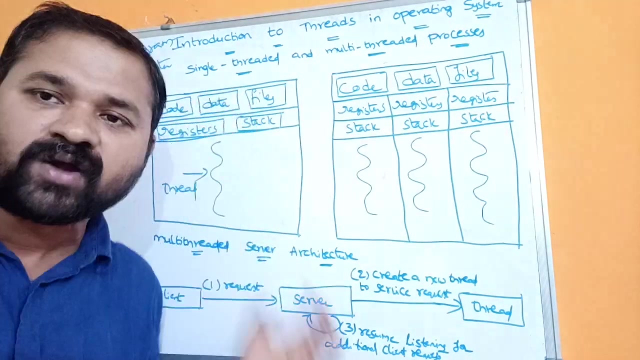 So stack section contains details about the function. So whenever we call the function, then all the parameters as well as local variables will be pushed down to the stack. Let's see the problem with. a single threaded process Assumes that this process is blocked. Now CPU has to wait until that process is unblocked. 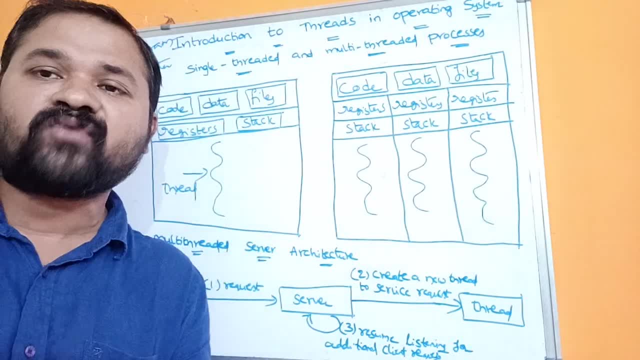 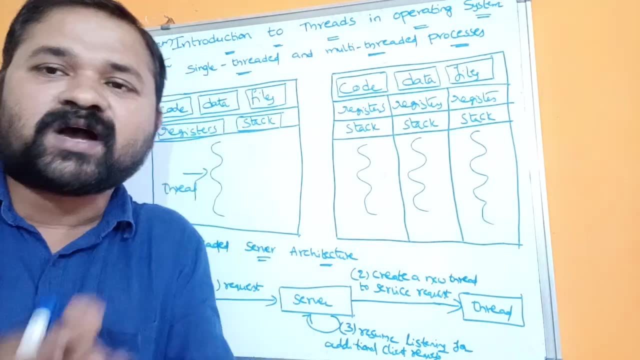 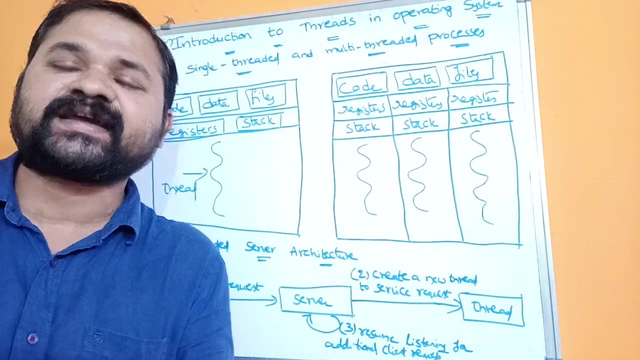 So for that CPU has to wait for a long amount of time. So in order to execute a single threaded process, CPU has to take more amount of time for its execution, Because whenever that process is blocked, then CPU has to wait until it is unblocked. 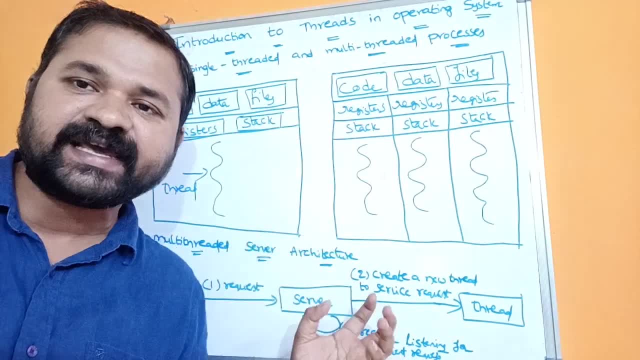 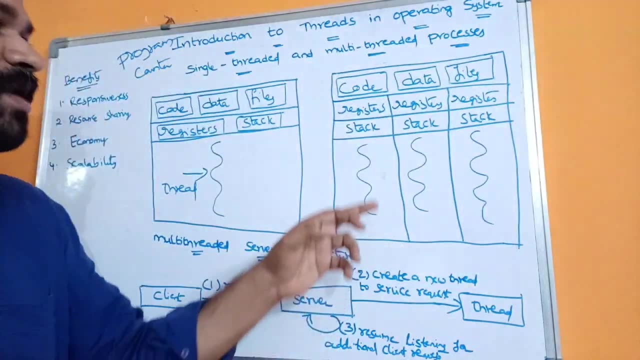 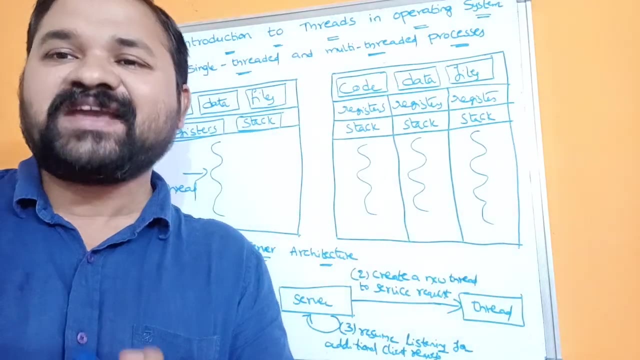 So the major problem with single threaded process is here. for execution, we require more amount of time. We can overcome this problem with the help of multi threaded programming. In multi threaded programming, what we will do is we will divide the process into several tasks, Where each task is known as a thread. 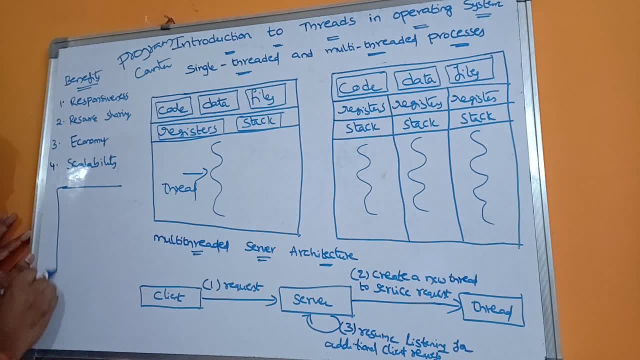 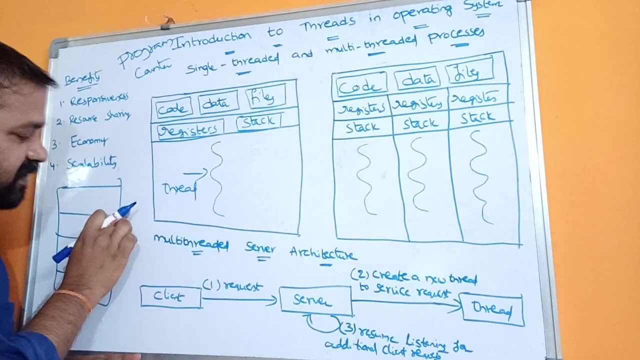 So let us assume that this is our process. So this process is divided into several tasks where each task represent a thread. So this is first task. So first task is nothing but thread 1.. Second task means thread. 2. Third task: thread 3.. 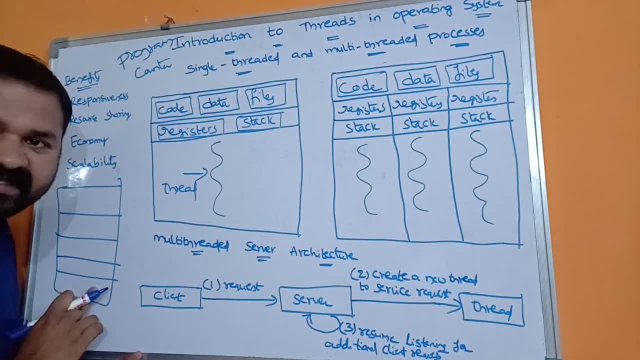 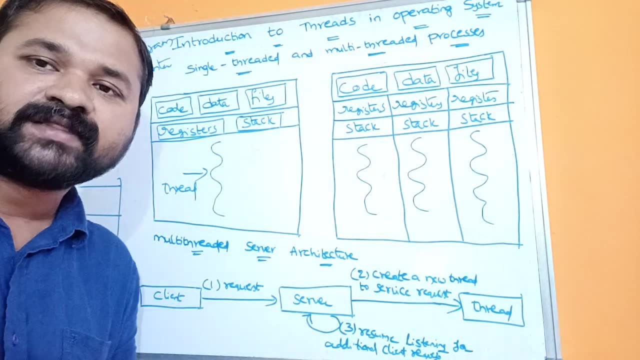 Fourth task thread: 4.. Fifth task thread: 5.. So if one thread is waiting for some blocking, So let us assume that one thread is waiting for blocking. So let us assume that one thread is waiting for some blocking. one thread is blocked, then cpu control will be shifted to the second thread. so cpu starts. 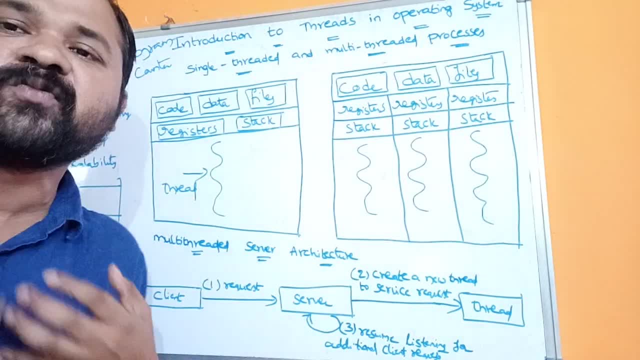 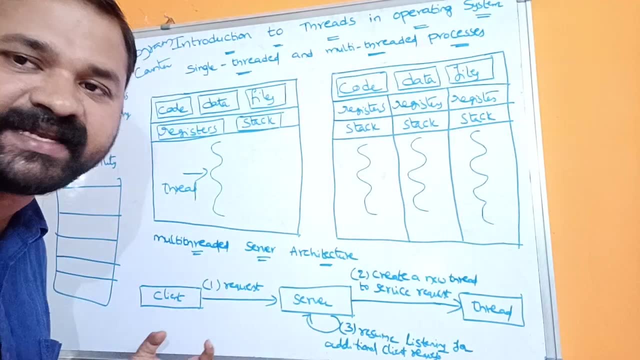 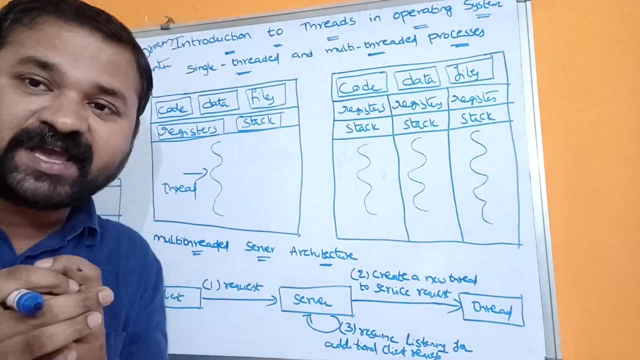 executing the second thread assumes that second thread is also blocked. then cpu control will be shifted to some other block, some other thread, so cpu starts executing the third thread. so likewise, most of the time cpu is executing this process. so with less amount of time we can execute that. 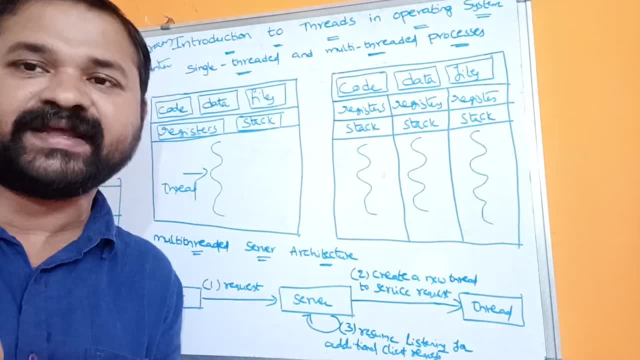 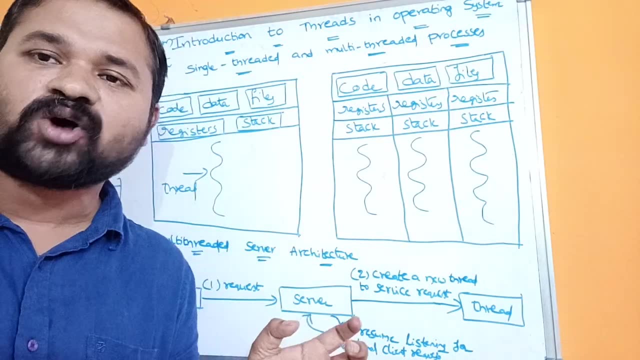 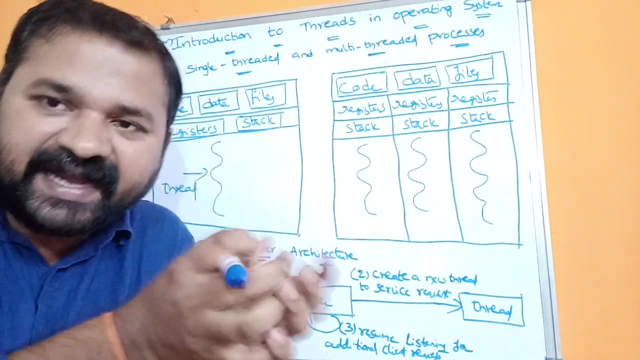 so we can get the output in a faster manner. so that is the advantage of multi-threaded programming. cpu will not sit as idle. why? because here we are dividing the process into several tasks, where each task represents a thread, so now we can execute all these threads simultaneously. concurrently, so with less amount of time we can get the output. so here the measured ありがとうございました. advantage of the multi-threaded programming is: it achieves concurrency, it achieves parallelism. why? because what we are doing, we are executing multiple threads simultaneously. okay, here there is no need to create separate address space for the thread. the thread will share the same address. 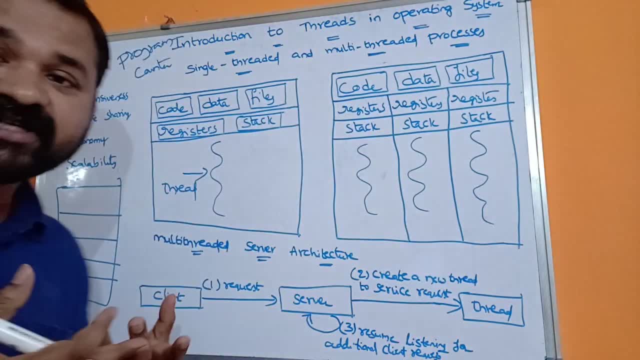 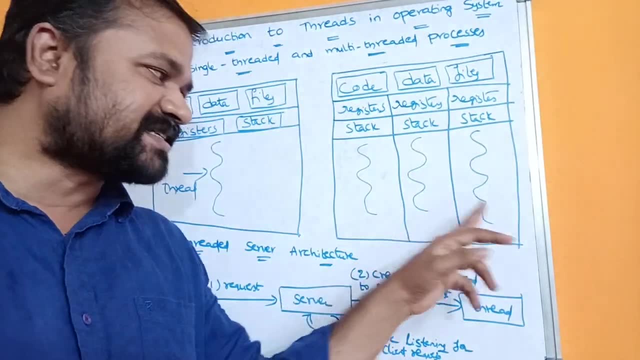 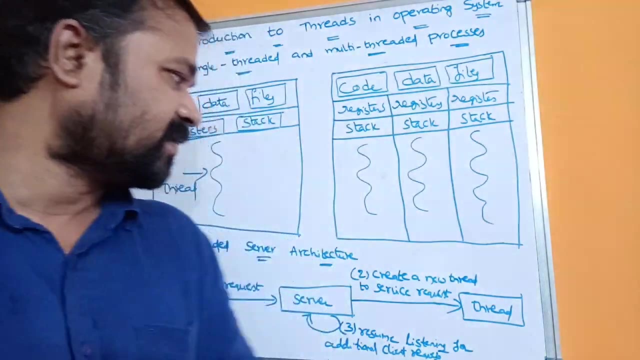 space of the process. okay, so that is the advantage of the multi-threaded programming. we will discuss more advantages here in benefits. let us see the sections here. here we have three threads, so these threads will defines the flow of execution. that means how those statements will get executed. so here we have three threads here. all the three threads are sharing the code. 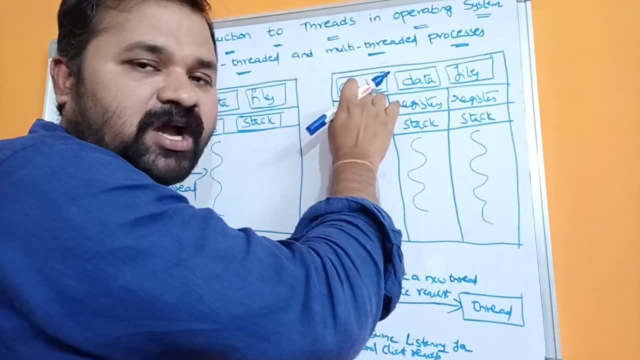 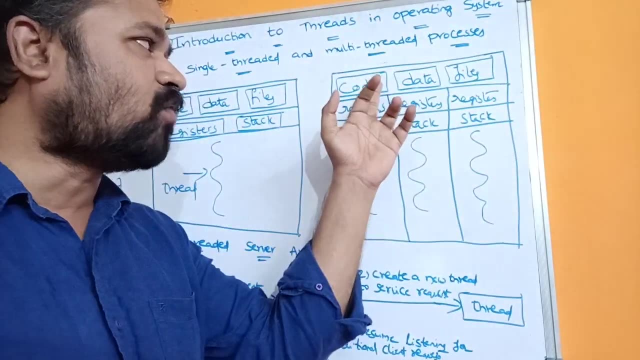 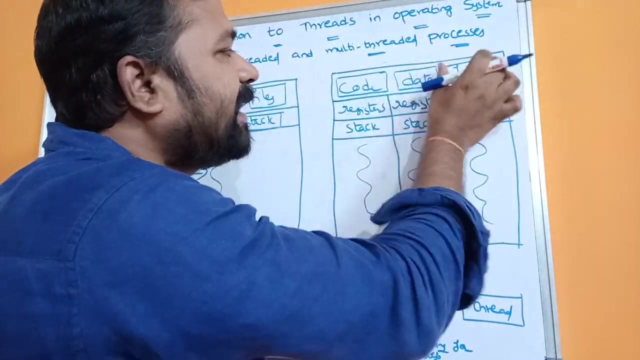 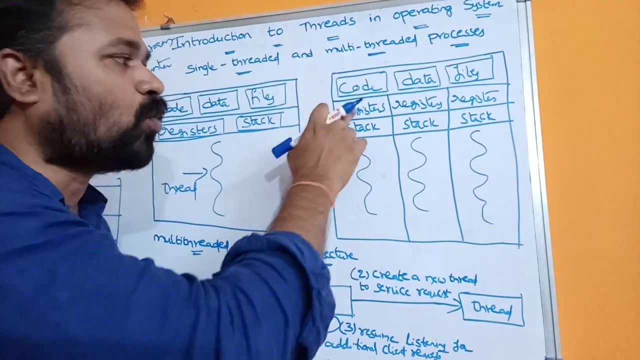 section, data section and file section. that means here the code section, data section and file section is same for all the threads. so we know what is code section, what is data section as well as what is file section. so here all the threads are sharing the same code section, same data section and same file section, whereas each thread has its own register. 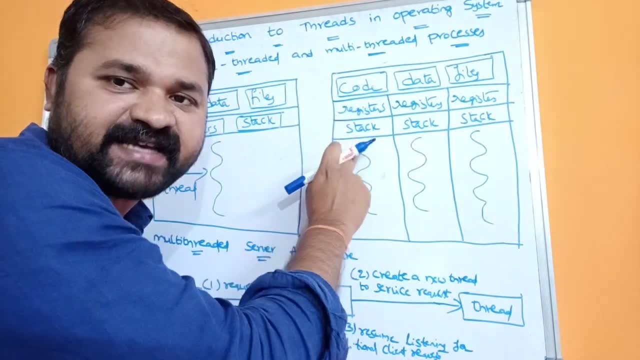 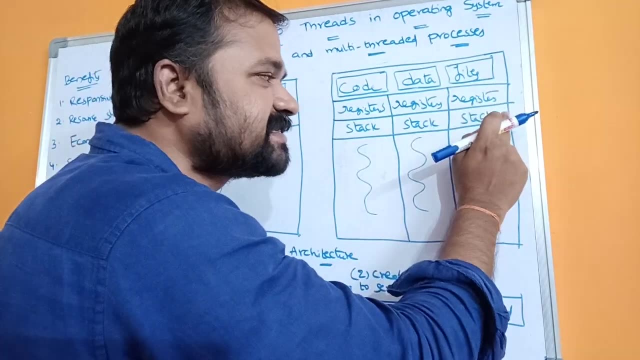 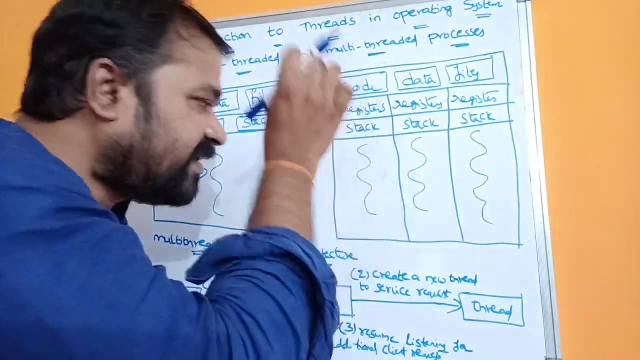 and stack. so thread one has its own registers and stack thread two. two has its own registers and stack 33 has its own registers as well as stack. okay, so each thread is having its won't register and it's won't stack. why? because whenever this thread is blocked, then we have to. 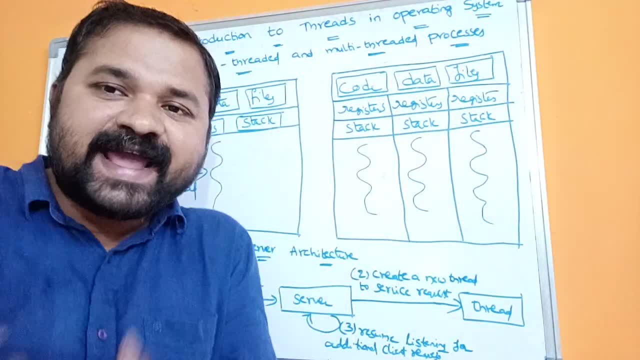 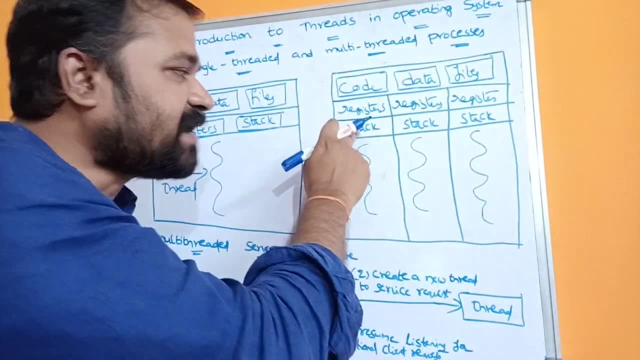 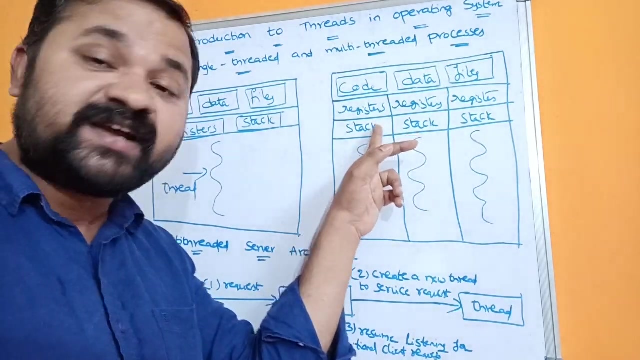 store thread one information- that means the next instruction of the threads- in its register only. we can't store in another register. okay, likewise in this thread. if we call any function, then that function information will be stored in thread one corresponding stack. we should not store thread one. 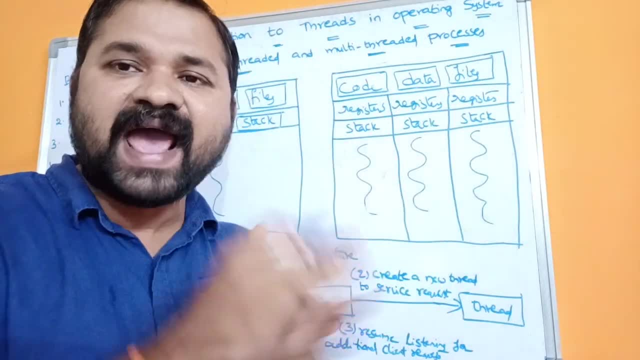 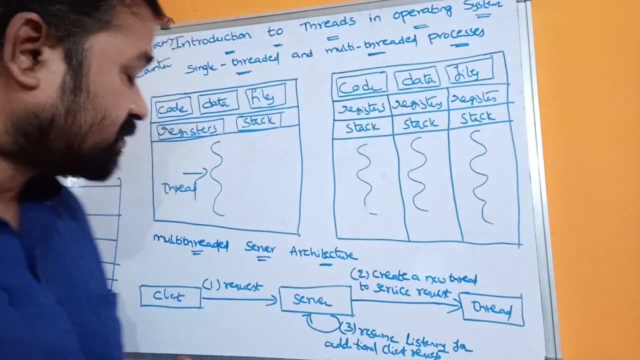 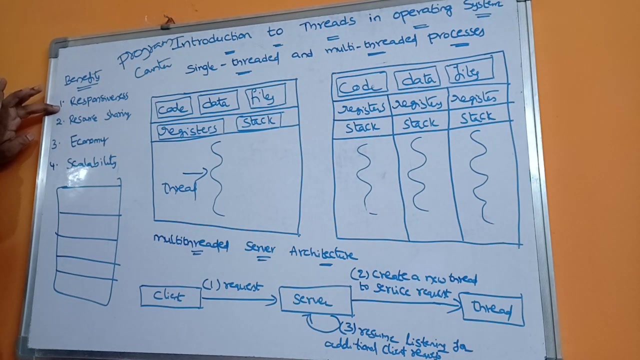 function information in 32 stack. if you store like that, then it will give the wrong results. so this is the. this is about what is multi-threaded process. now let's see about the benefits of multi-threaded programming here. mainly, there are four benefits are there? first one is responsiveness. 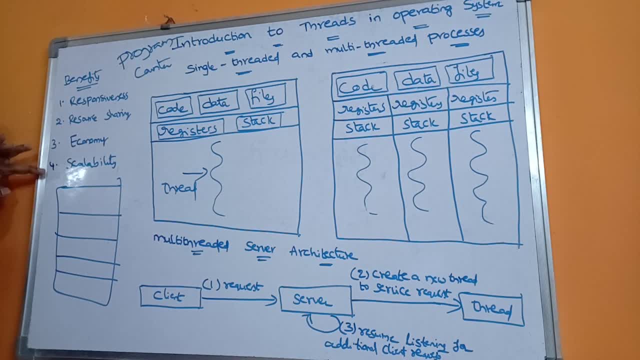 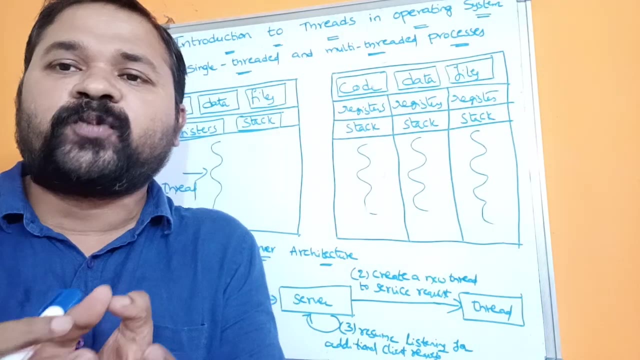 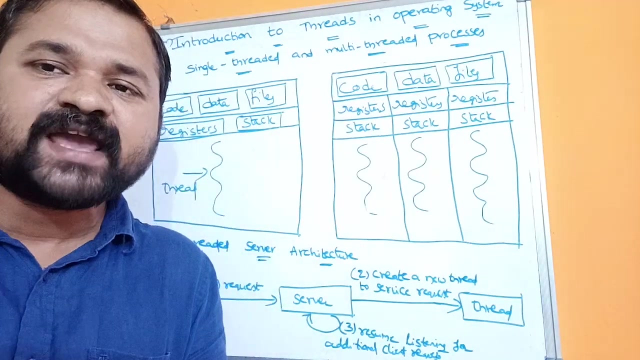 second one is resource sharing. third one is economy. fourth one is scalability. so these four are the benefits of multi-threaded programming. let's see all these benefits by one. first one is responsiveness. responsiveness means here it will gives the output in a smaller amount of time. the response time is very, very fast. so why response time is fast in multi-threaded? 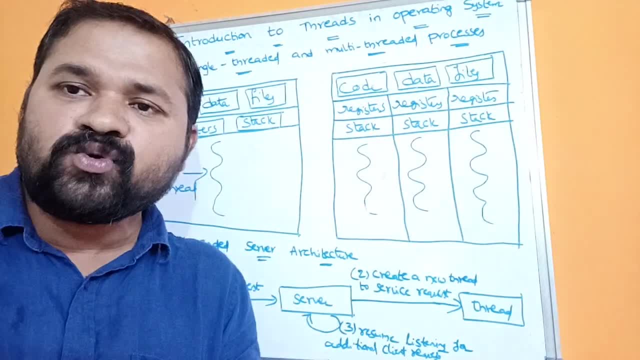 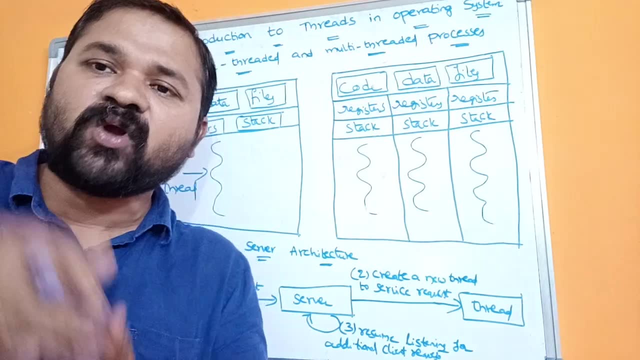 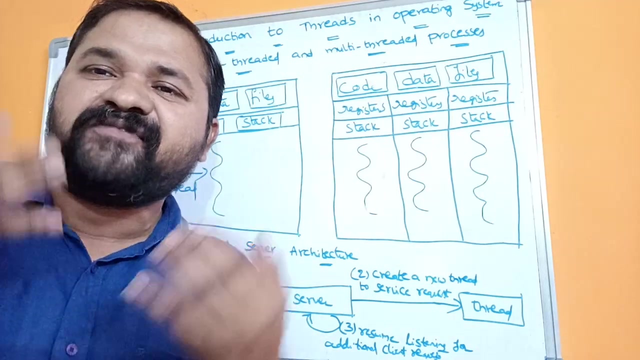 programming. if one thread is blocked, then cpu control will be shifted to some other threads, so cpu starts executing the threads, suppose. if the second thread is also blocked, then cpu control will be shifted to the third rate. so here we are using the cpu in efficient manner by switching between the threads, so with less. 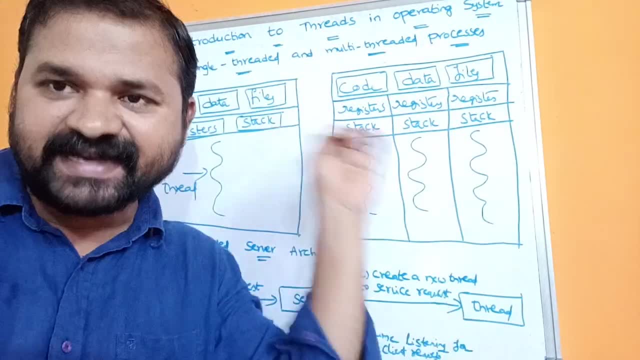 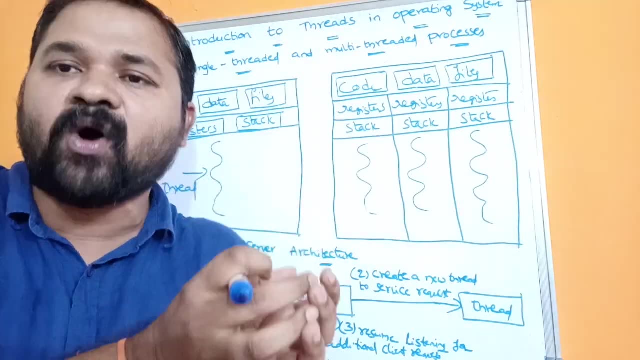 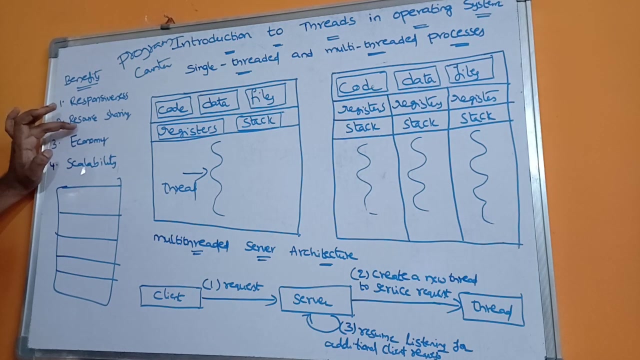 amount of time cpu will produce the output. so that is the first advantage: responsiveness. here the response is very, very fast. the response is very, very small. in less amount of time cpu produces the output. let's see the second advantage of the multi-threaded process. the second advantage is: 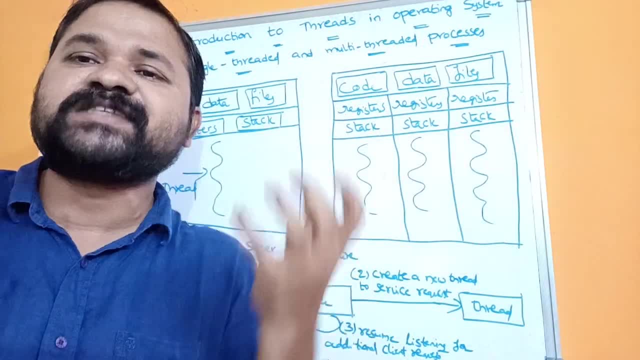 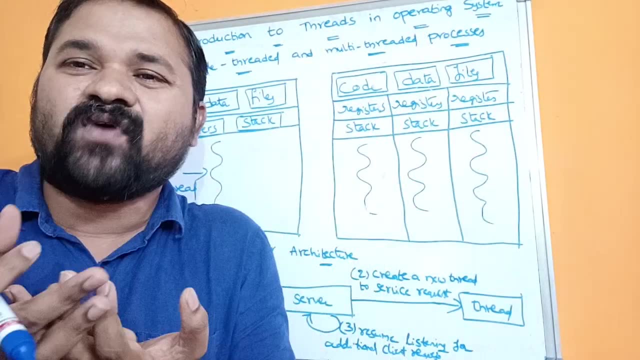 resource sharing. here the sharing of the multi-threaded process is very important. here the sharing of the resources is very, very easy. why? because here all the threads are using the same data section. let us assume that we want to use a global variable. so then what will happen? so we can. 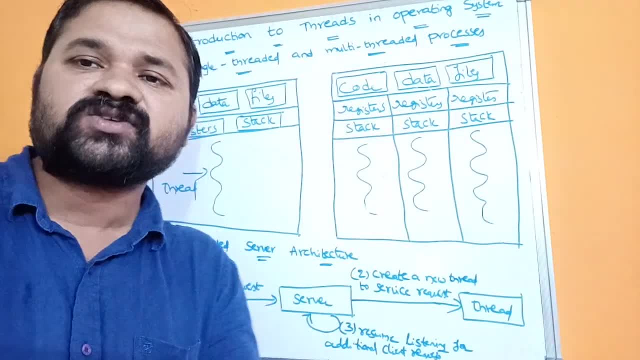 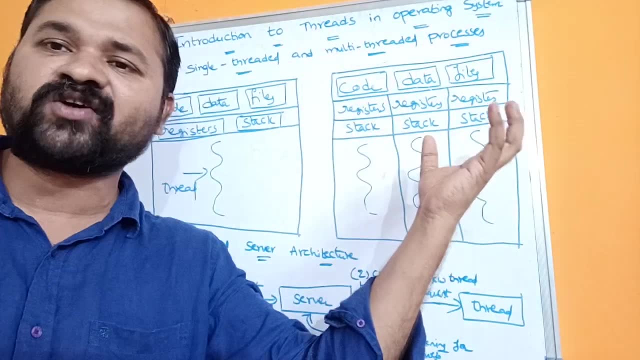 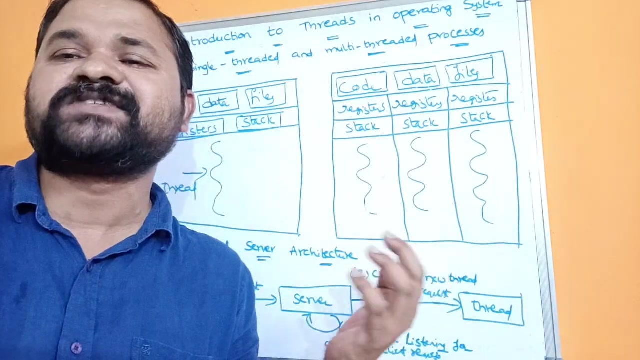 use that global variable throughout the program very, very easily. so one thread can read the data from the global variable. another thread will write, will do some modification on the global variable. so it is very, very easy. so resource sharing in multi-threading, multi-threaded process is 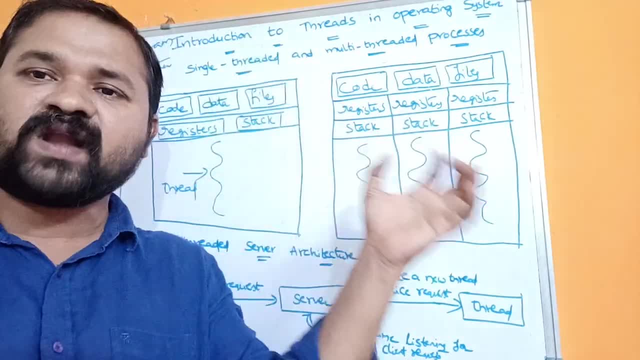 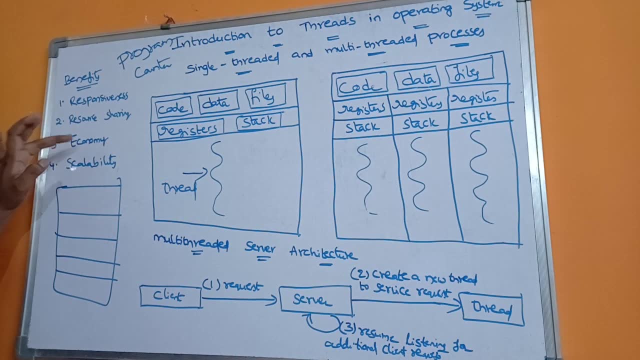 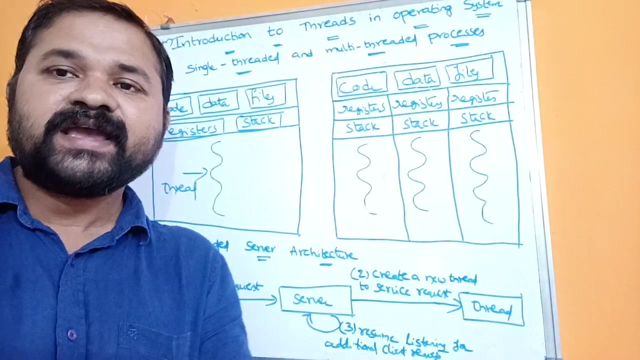 very, very easy. simply by making use of the global variable we can share any resource in an easy manner. and the third one is economy. so multi-threaded process is very, very cheaper when compared with the multi-processes. here we have multiple threads. creating the thread is very, very. 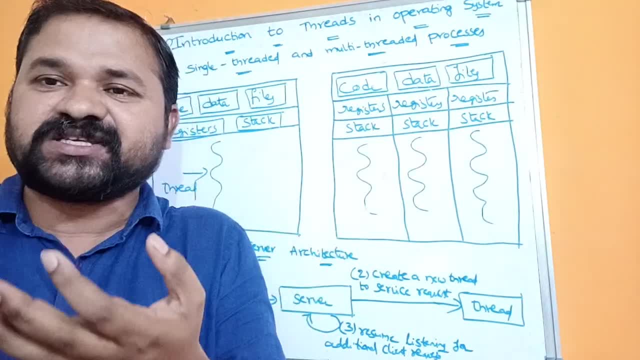 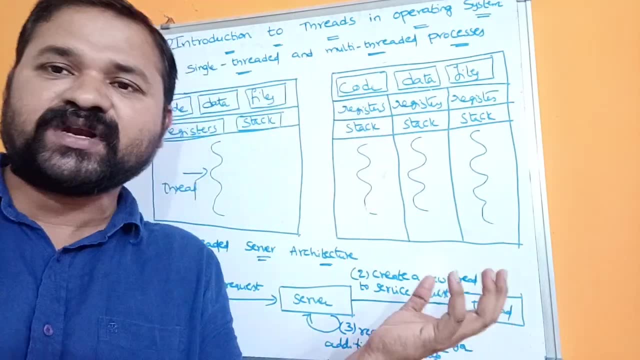 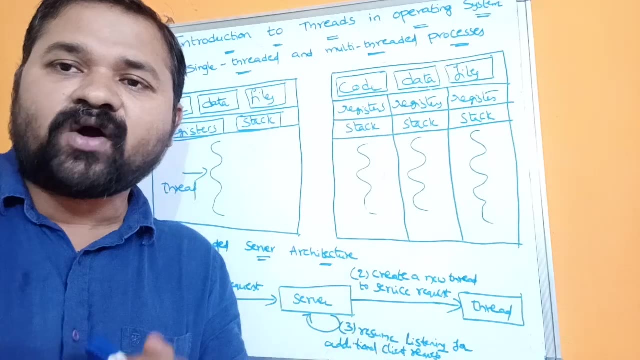 cheaper, as well as very, very, very, very inexpensive. okay why? because thread doesn't require additional data, so it is very, very cheap and it uses the address space of the process only, as well. as context switching of the threads is very, very easy, very, very faster. we know what is context switching. 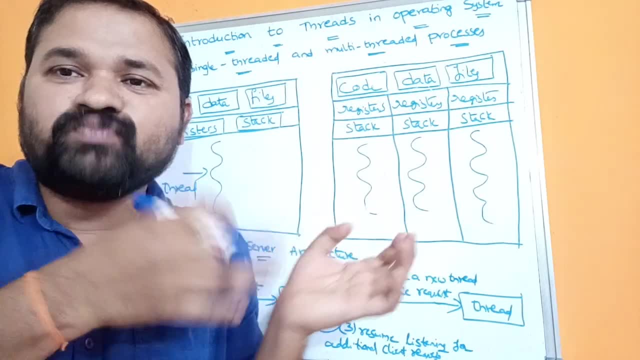 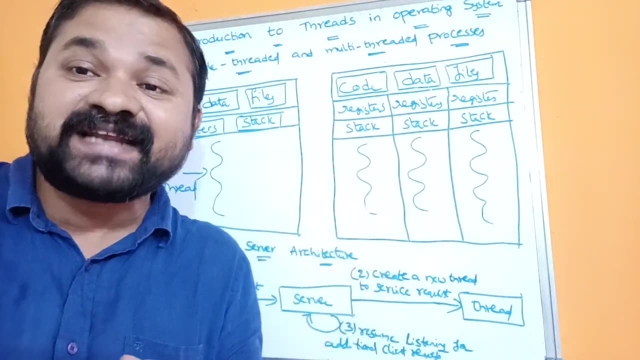 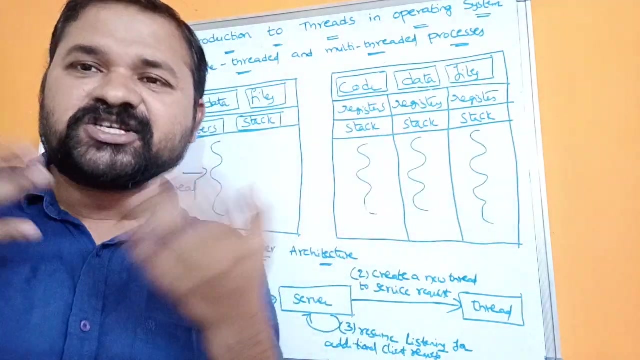 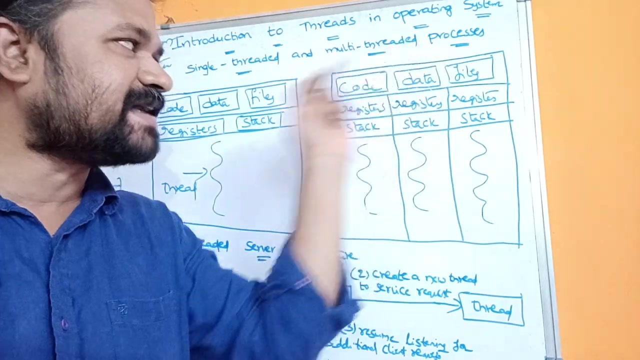 switching between multiple threads here. here all the threads are belonging to the same address space, so switching from one thread to another thread is very, very faster, as well, as inter-thread communication is very, very fast. here there is no need to use inter-process communication mechanisms like rpcs, sockets- all those are not needed here. okay, simply by making use of this data section. 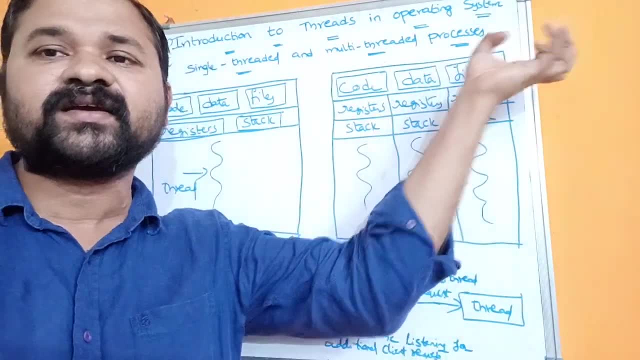 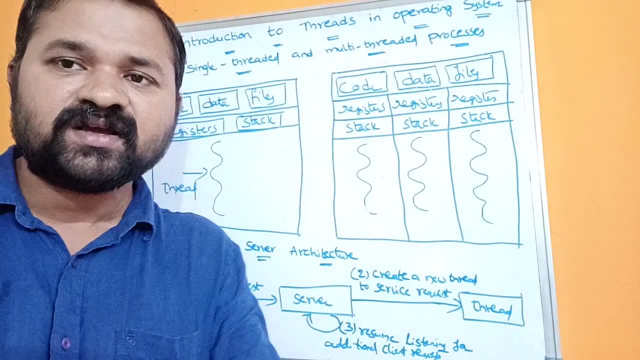 one thread can communicate with another thread very, very easily. if one thread wants to give some data to the another, threat that the thread places that corresponding data in data section so another thread can access the data in a faster manner. so we can say that multi-threaded process. 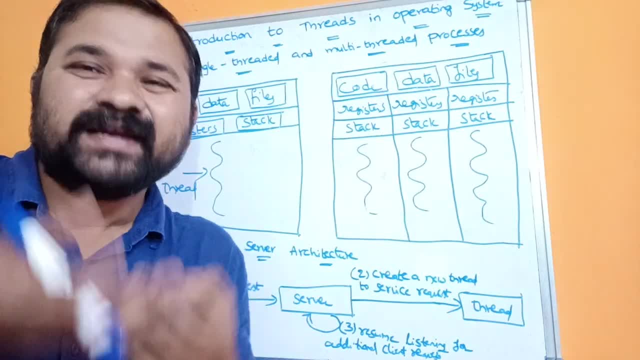 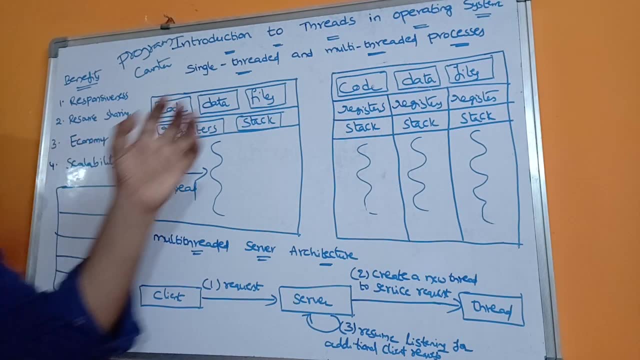 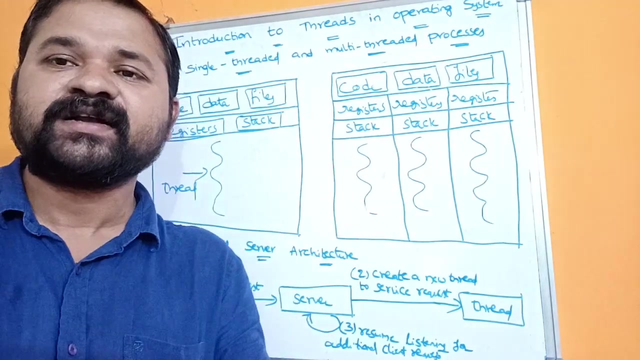 is very, very less economy. okay, it is not an expensive process. it is very, very cheaper. and the last one is scalability. here we can extend multi-threaded process to the multi-processor architecture, so we know what is multi-processor instead of having a single processor. 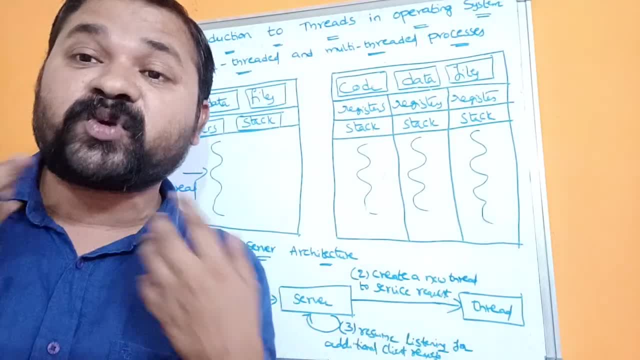 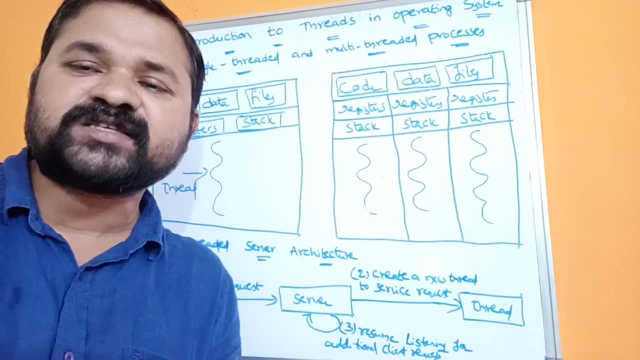 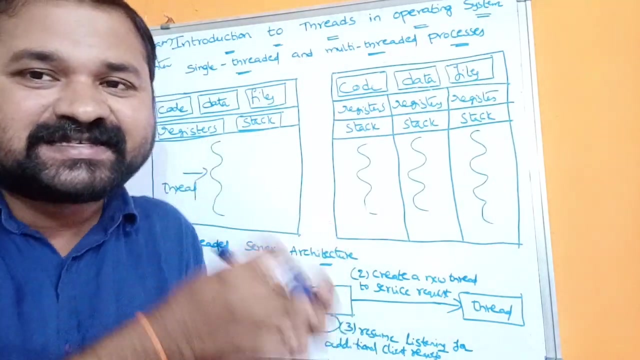 we can make use of multiple processors. let there are three processors in the system where the first processor will execute thread one. second processor executes thread two. third processor executes thread three. so in very, very less amount of time we can get the output. so we can extend. we can scale this to multi-processor architecture so with less time we can produce.